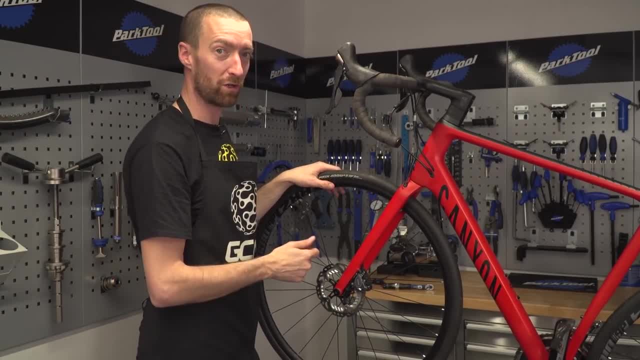 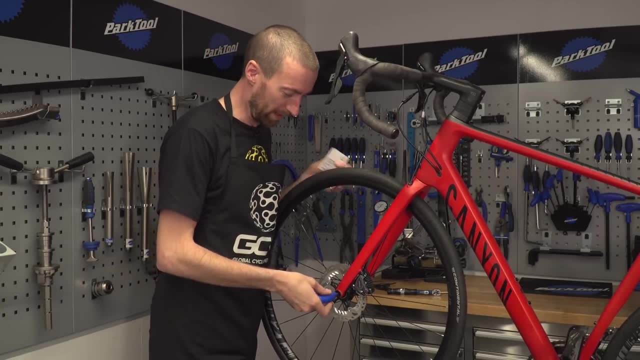 But with flat mount discs in particular, it can be a little bit more complicated. Now for the hack. you are going to need some kind of business card- I've taken one of Si Richardson's- and you're also going to need to take the wheel out, which, for this particular bike, is a six mil. 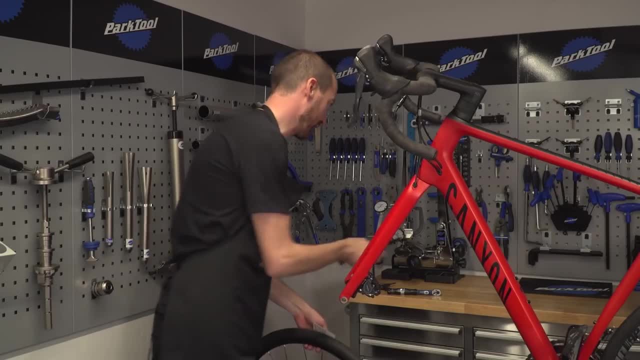 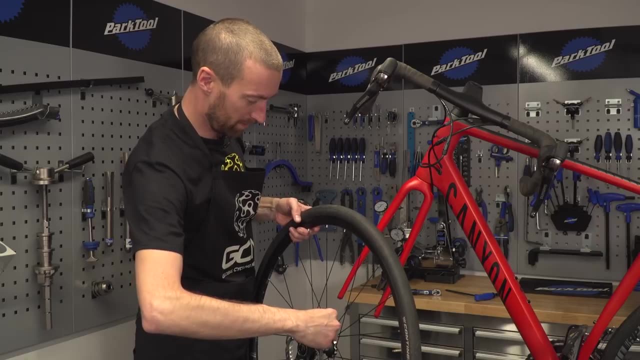 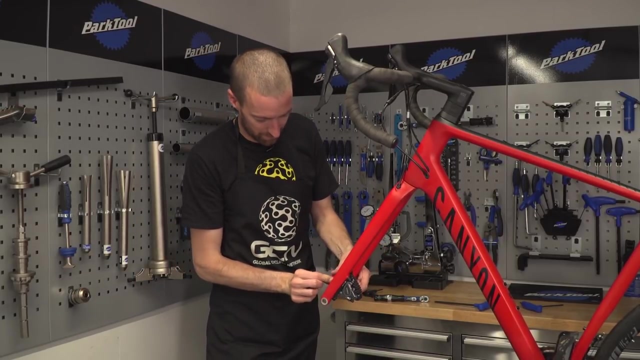 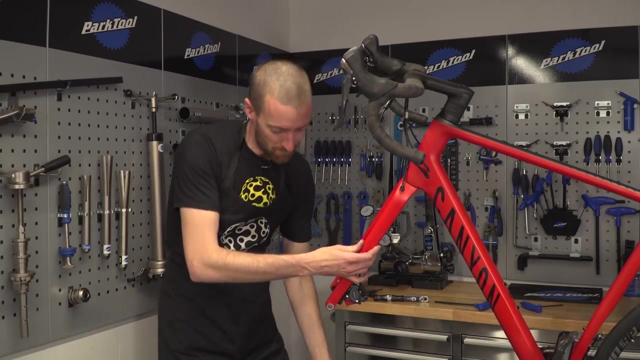 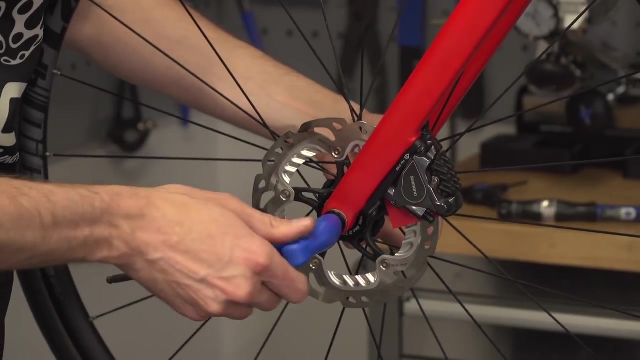 Allen key. Drop it out briefly. Then you're going to take your business card and bend it over the rotor like so, And once you've bent your card into shape, insert it into the caliper, then put your wheel back in. Then we are going to loosen. 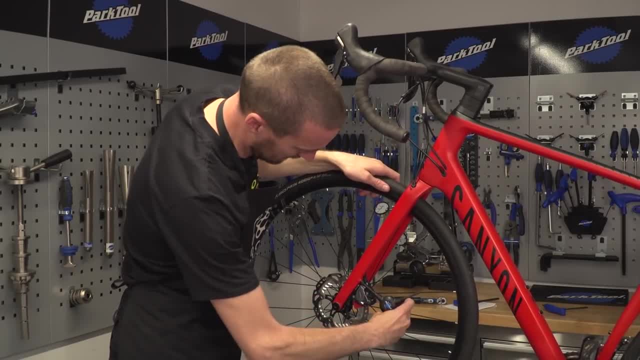 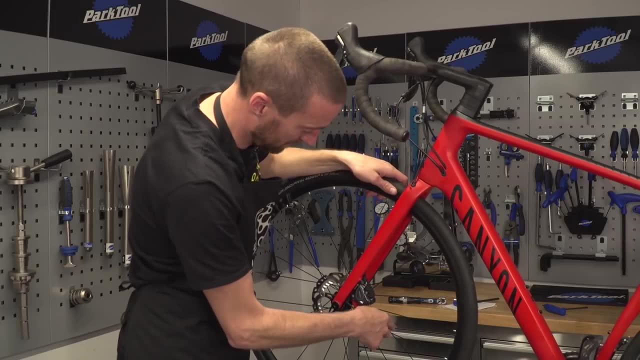 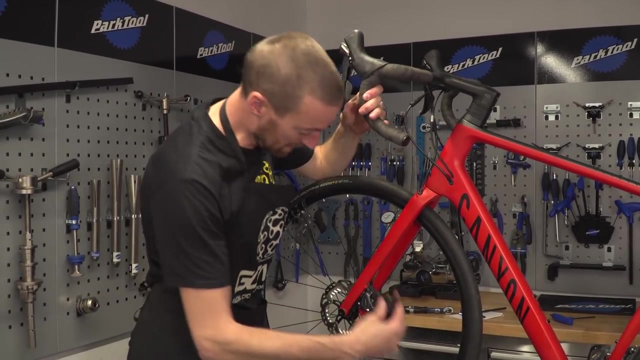 the caliper off again, as we did before, And the width of that business card should be just the right size to space the pads out nicely. So pull your brake on again. Should be all nice and centered And then you can do it back up. 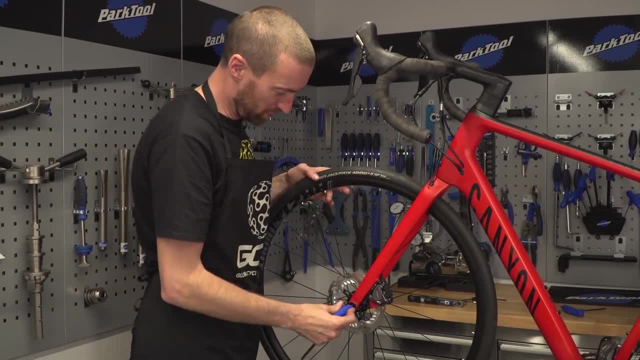 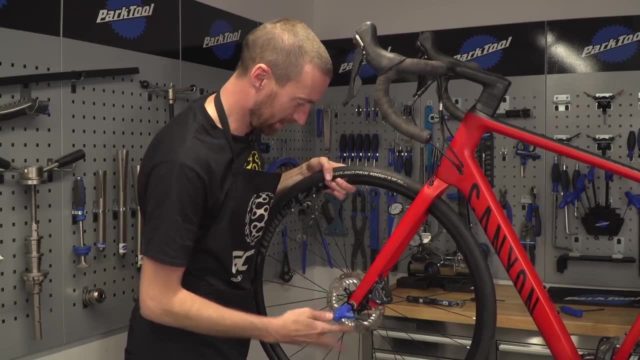 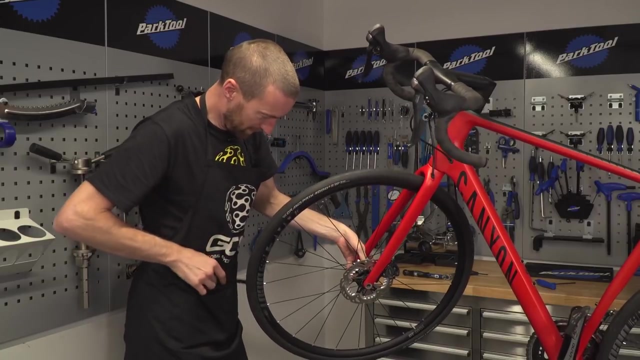 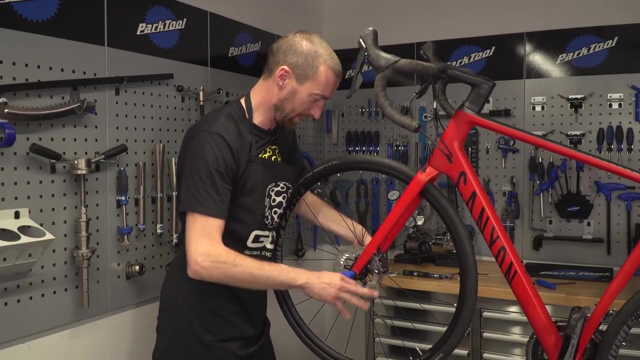 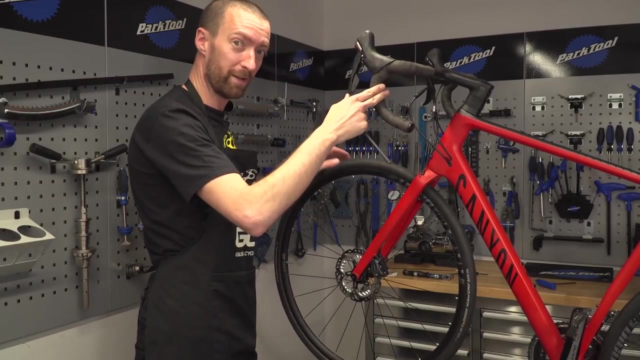 with your torque wrench again. Then you are ready to drop the wheel back out again and remove your business card And then hopefully everything goes perfectly And you put your front wheel back in and tighten the whole lot up. Everything should be perfectly centered and no sign of any disc rub. Perfect disc brake hack. 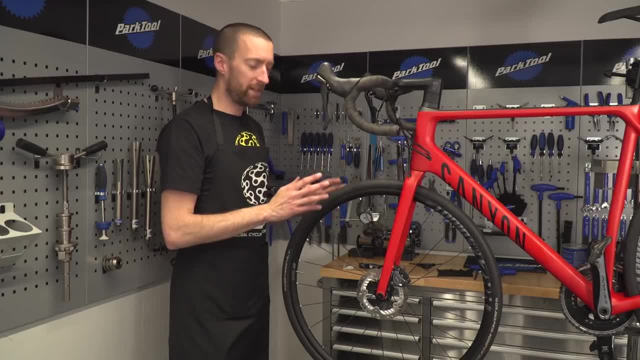 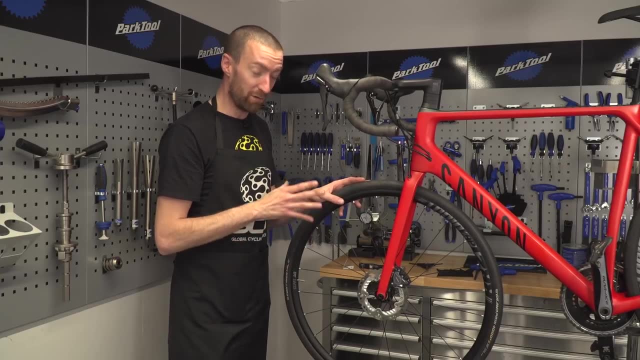 pa. Now it's fair to say that for the majority of us, disc brakes are relatively maintenance free, and that is a fair reputation. but if you ride a lot in bad weather, there is something else that you need to know about and be aware of, and that is sticky pistons. 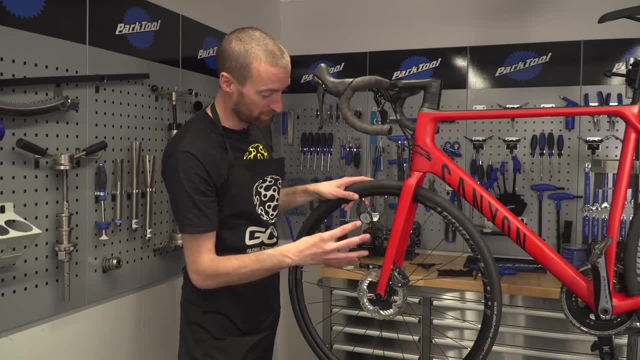 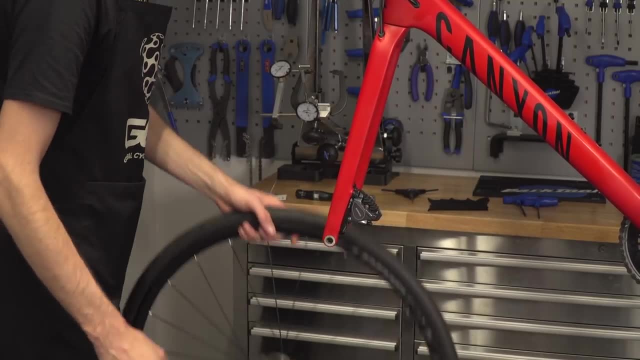 Now, the pistons are essentially what's inside the caliper here, which pushes the brake pad onto the rotor, and they can occasionally become sticky. They're in their own little oil bath and you'll be able to tell by looking inside them. 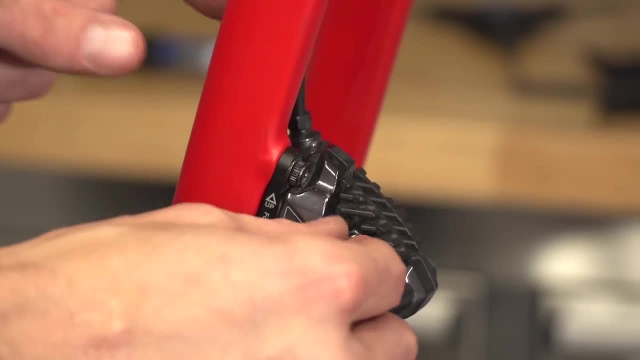 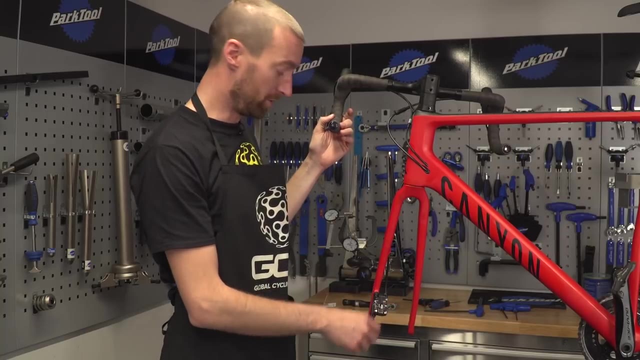 It won't necessarily be evident just by pulling the brake lever on here. So to get access to them you'll need to remove the wheel and also remove the brake pads. Then, once you've got the pads removed and the pistons exposed, you want to pump the brake. 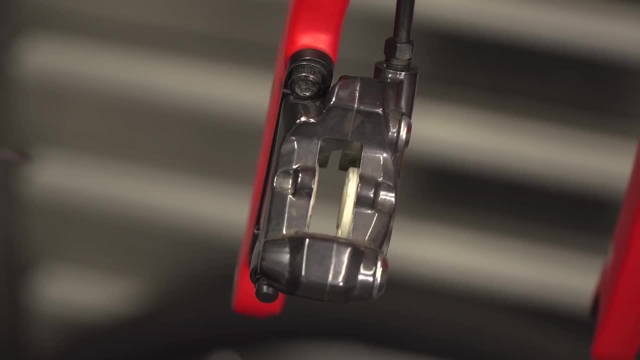 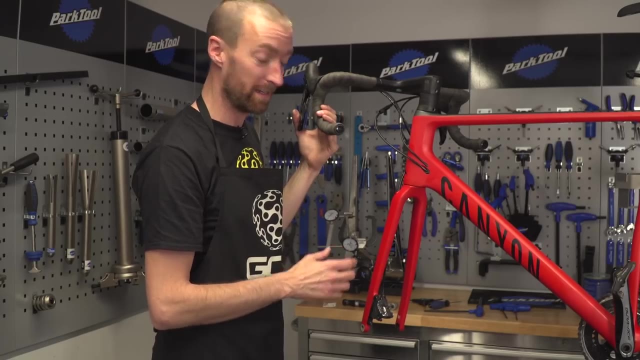 lever a few times to pop them slightly out. Make sure you don't go over the top when you're doing this, because it is very easy to pop the pistons out completely and that will mean a full re-bleed. So just do it a few times until you've got around three or four millimeters exposed. 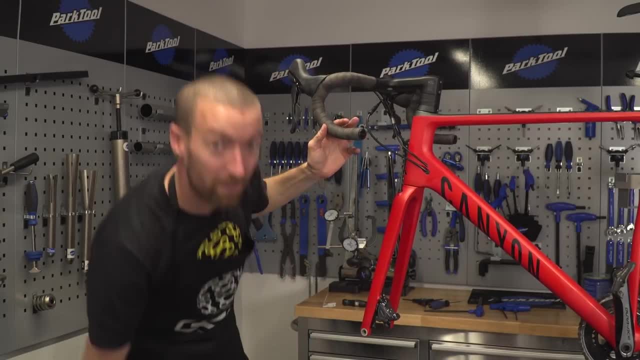 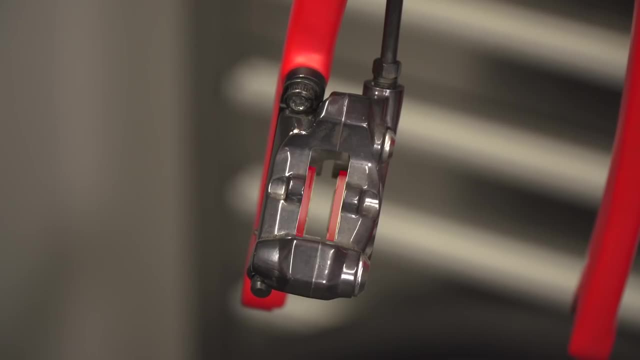 on both sides, At which point you want to get yourself some alcohol spray and a nice clean rag and clean the non-pad-facing side of the piston so effectively- the bit that's around the edge. that needs to be nice and clean when it's going in and out. 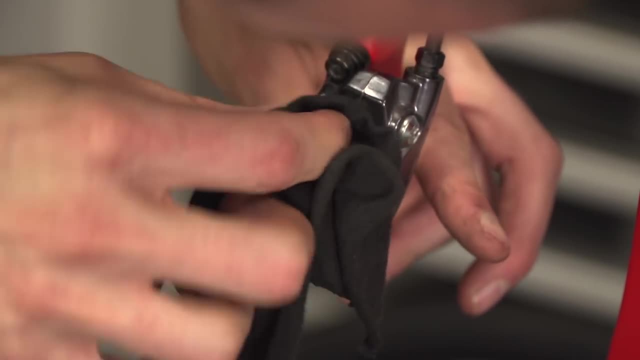 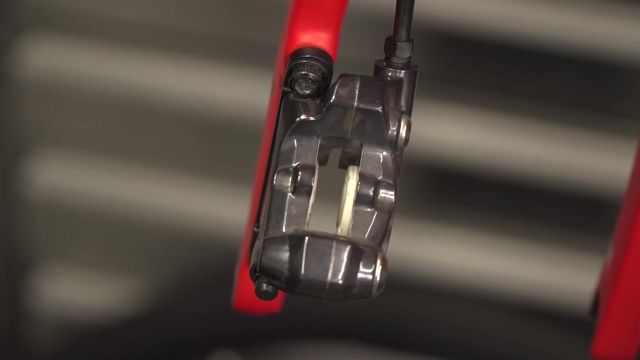 Now, if one piston is particularly sticky, what you might find is that the other piston has come out and is exposed, but one is left hidden, And in that situation, what you want to do is take the other piston, and you want to. 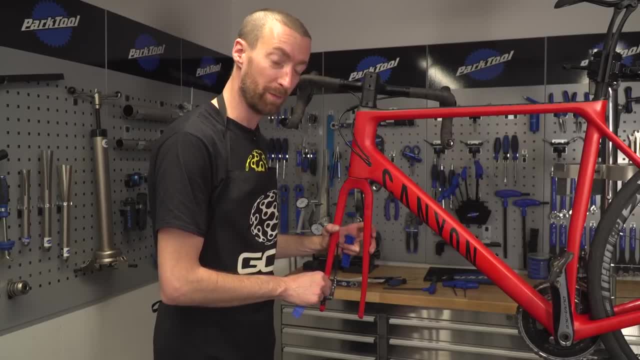 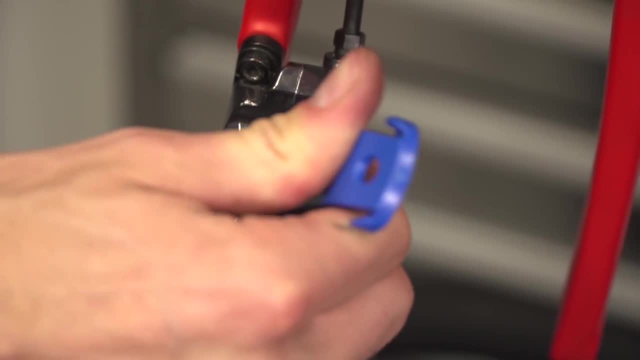 get rid of it, And in that situation, what you want to do is spend the first part of your time cleaning the exposed piston and then, using something like a plastic tire lever, push that one back in and then, with the fluid that's in the system, it should be enough to push the slightly. 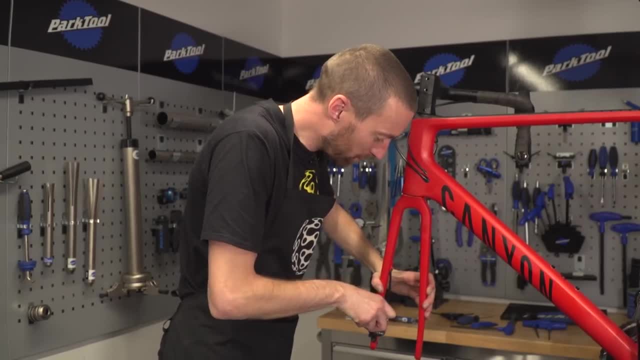 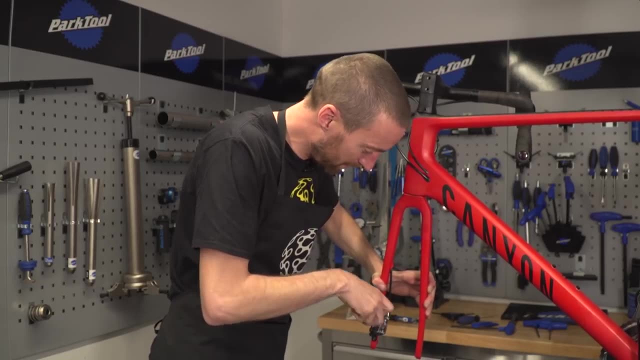 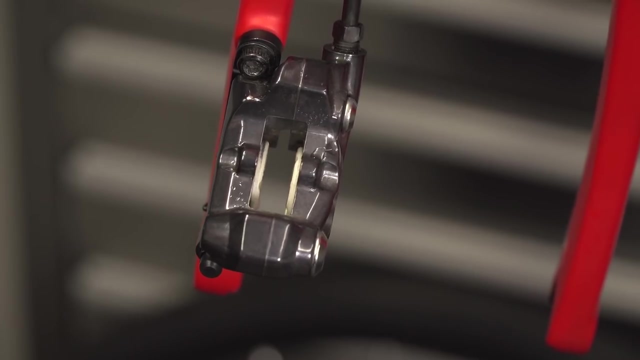 sticky piston out. Then, once they're all cleaned and dried, push the pistons back inside the caliper using a plastic tire lever and then give the brake a few pumps, just to check that they're now moving out nicely. Nice and evenly. 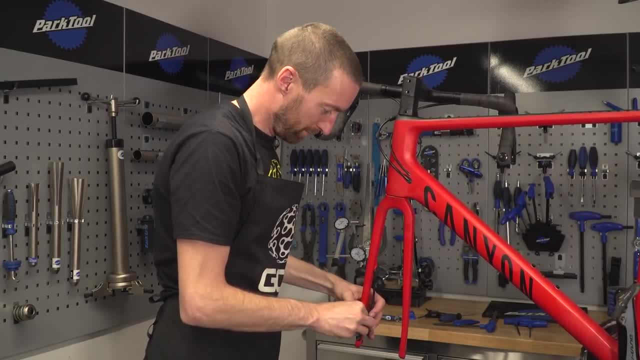 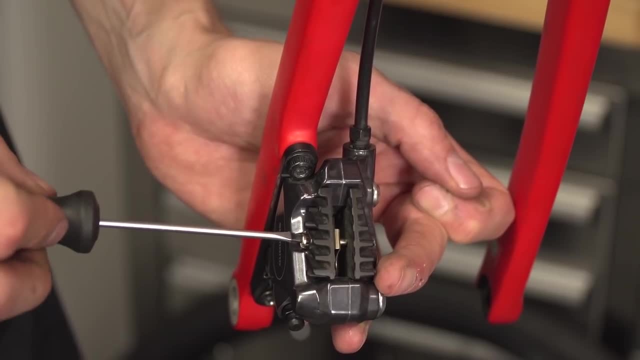 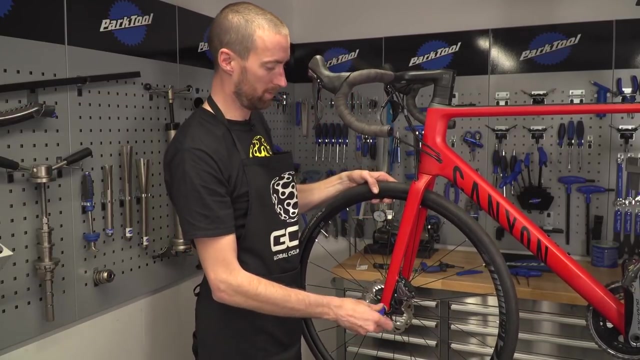 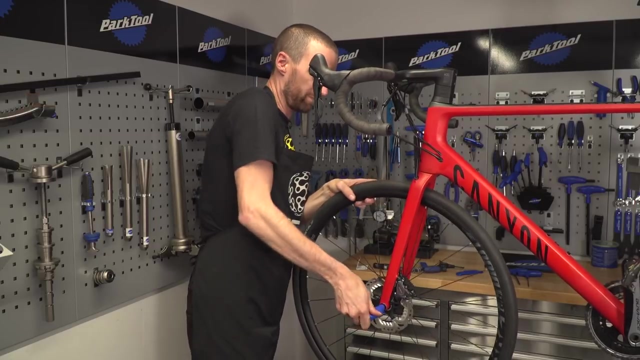 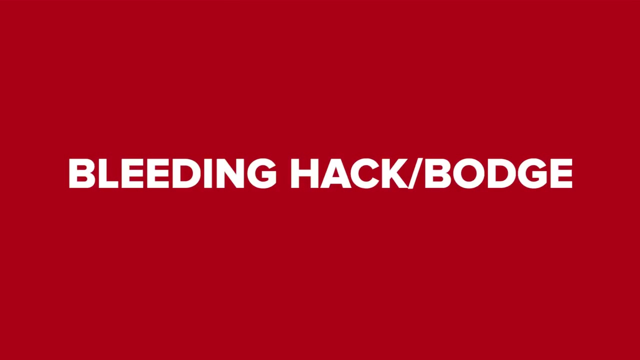 Then you just need to put the brake pads back in like so, and hopefully that will have solved your problem, And then stick your wheel back in. Looks nice and aligned already. Perfect Right. Next up is a hack which comes from our very own GCN mechanic, Tom. 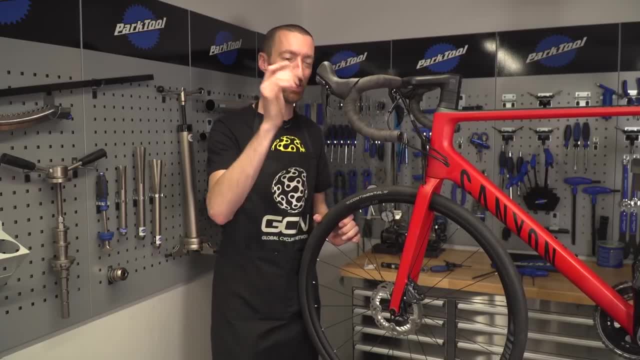 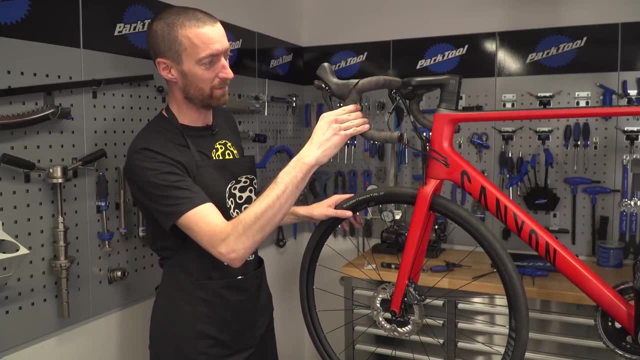 Not Tom Last, you understand, but somebody who actually knows what they're talking about. So if your brakes are starting to feel a bit spongy, ie from the first point of contact with the pad at the rotor, you can then pull the brake lever on significantly further. 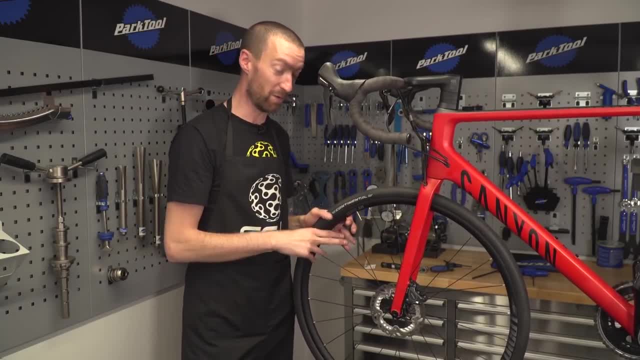 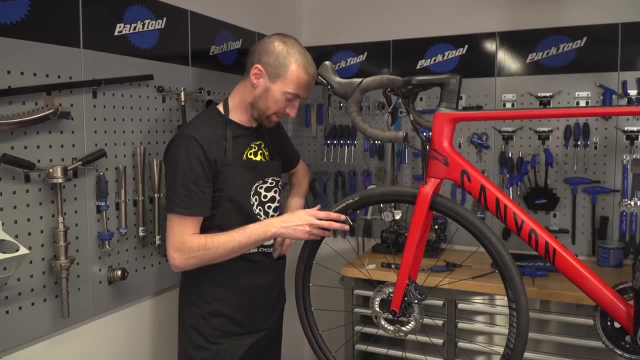 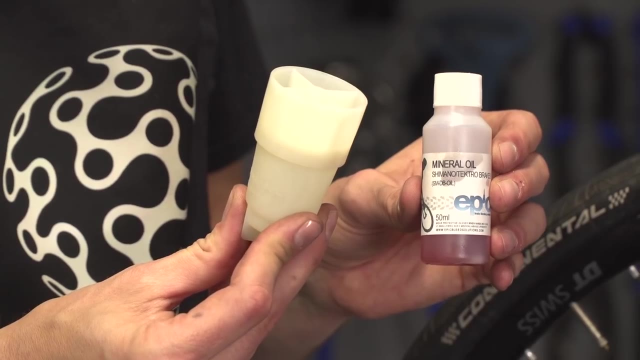 then it might be that the whole system needs to be re-bled, which is quite a big job. However, fairly recently, you might want to check this next hack out. for it, you are going to need a bleed bucket and also some fluid which is specific to your brakes. 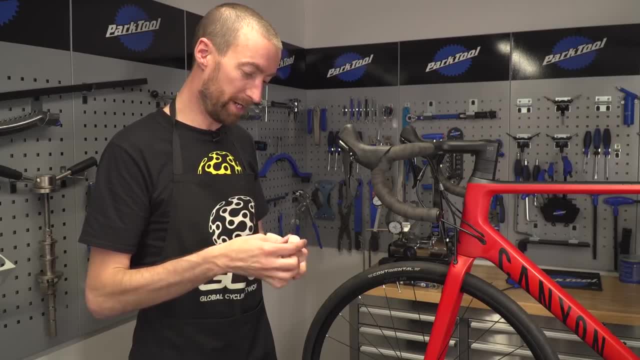 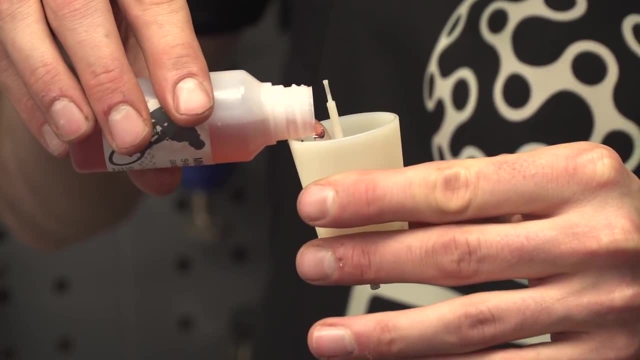 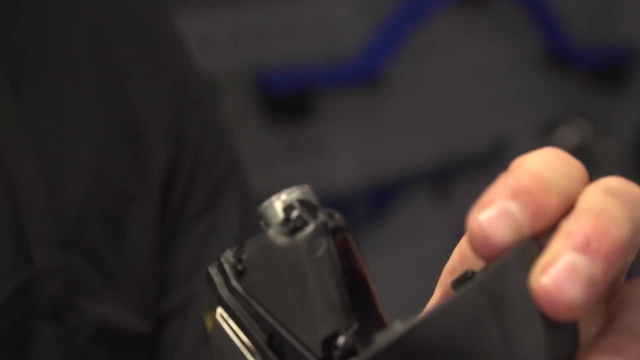 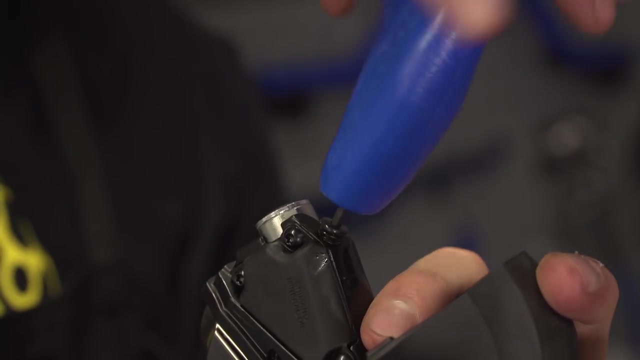 first up. you're going to want to put your brake specific fluid into the bleed bucket, fill it up around about a third and then put that to one side. then I want to expose the bleed port screw, which will be underneath the rubber hood here, and undo that. it's a two and a half millimeter allen key on this Shimano. 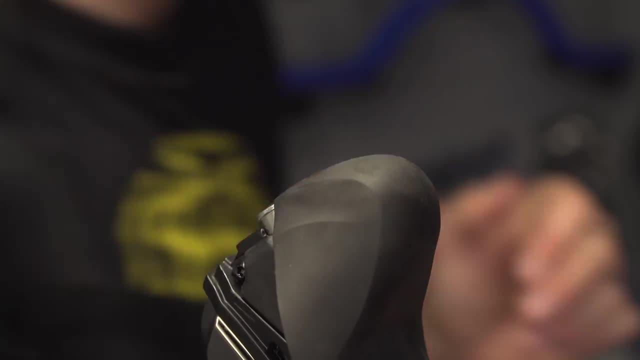 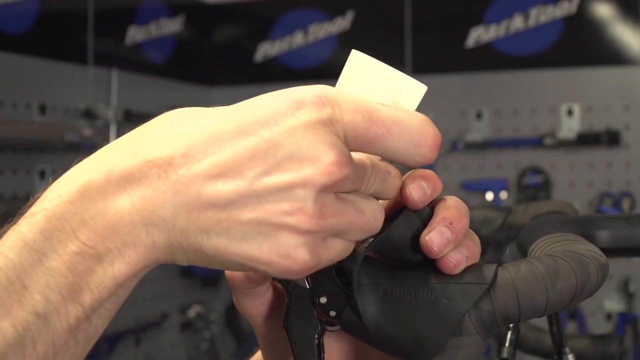 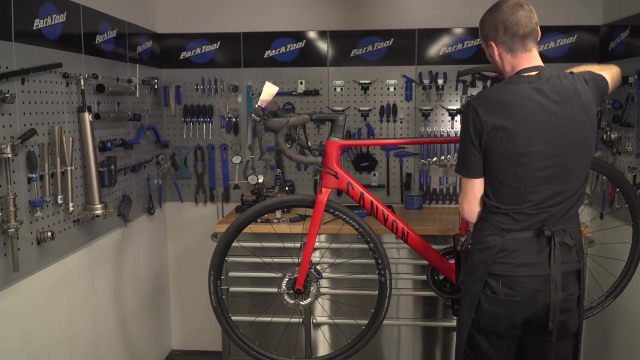 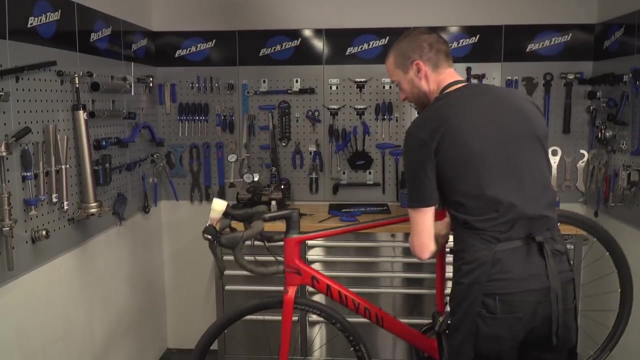 brake, pull that out, put it carefully to one side and then screw bleed bucket in right and then to do the actual hack part of this, we're going to take this, the bike, out of the stand, put it on the floor right, then take the top of the. 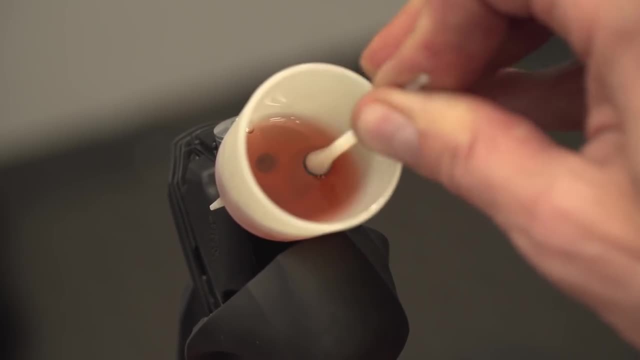 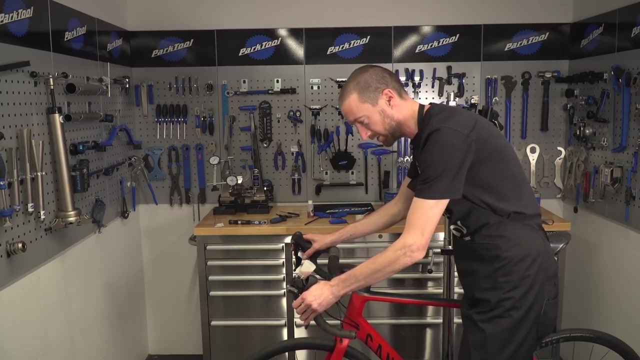 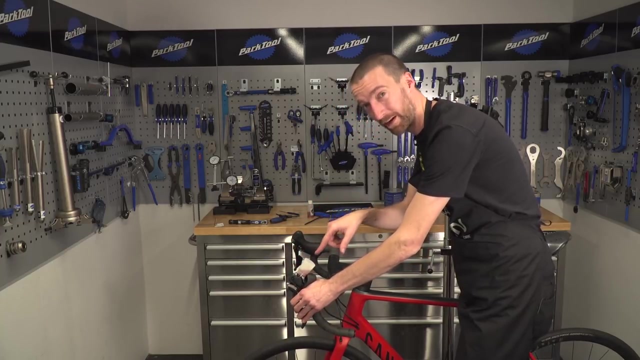 bleed bucket off and remove this plunger from inside. now squeeze the brake lever on and off a few times, do it as tight as you can, and what you should be encouraging is any air in the system to be coming up towards the top, and you might, in fact, see a couple of bubbles coming through. 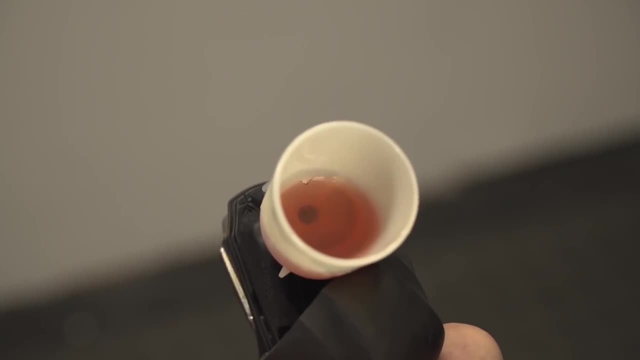 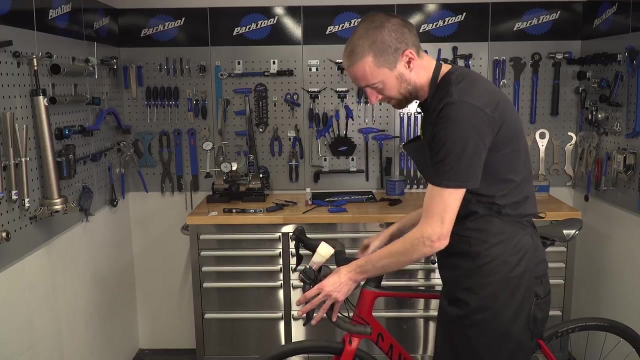 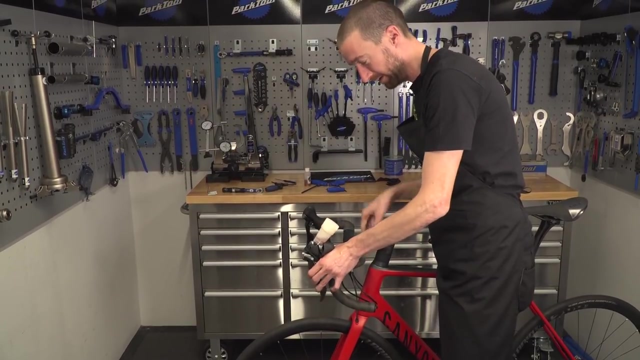 the fluid in the bleed bucket there. now, here's the extra little hack bit, though: take the top half of the bleed bucket and replace it, and then just gently squeeze the brake, whilst also gently tapping the front wheel up and down on the floor, and that will give an extra bit of encouragement to any air which is 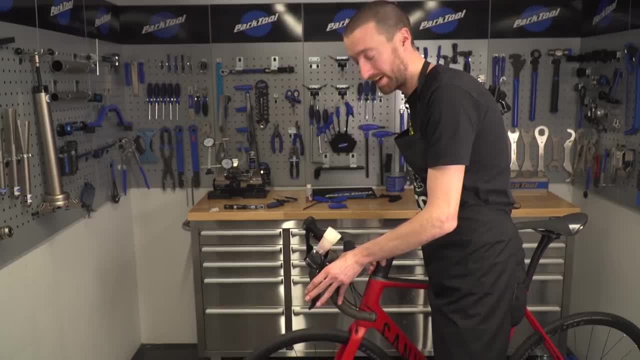 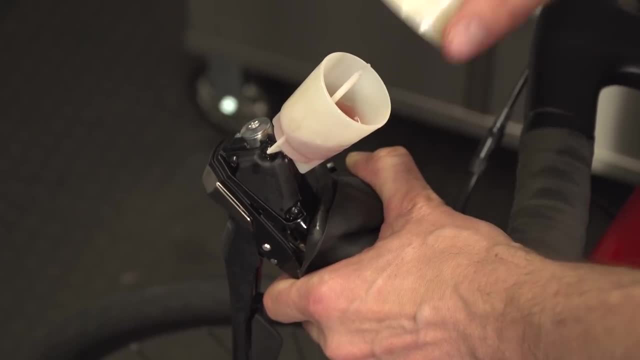 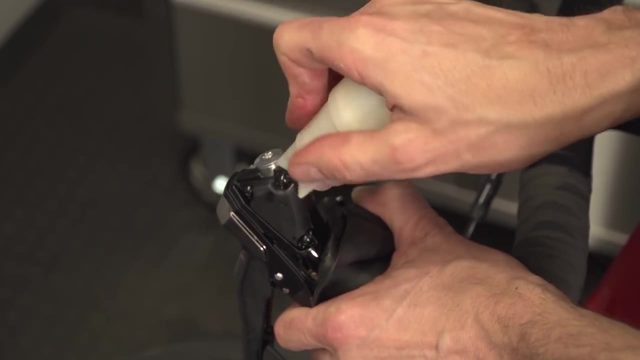 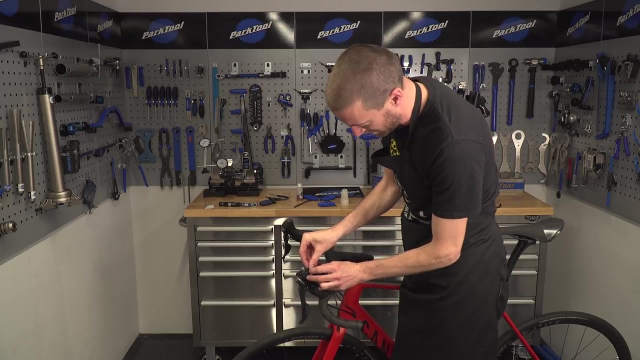 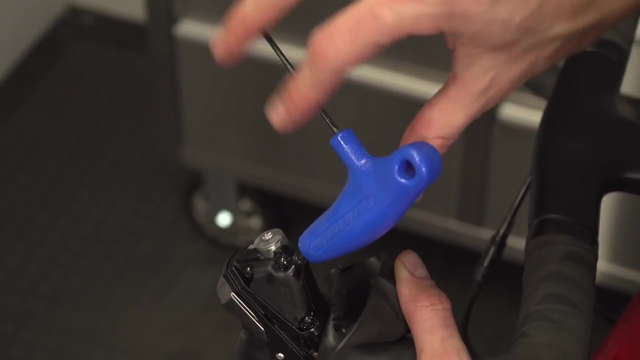 trapped in the system, which could well be the cause of your spongy feeling brakes, and hopefully that will have solved your problem. don't forget, though, to put the plunger back in before you unscrew the bleed bucket, otherwise you're going to get fluid everywhere. right then, back on with the screw, give everything a quick. 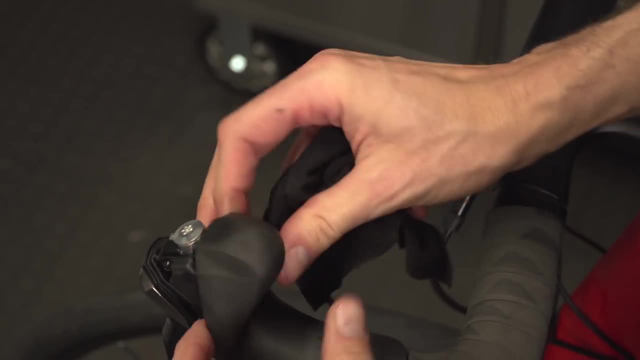 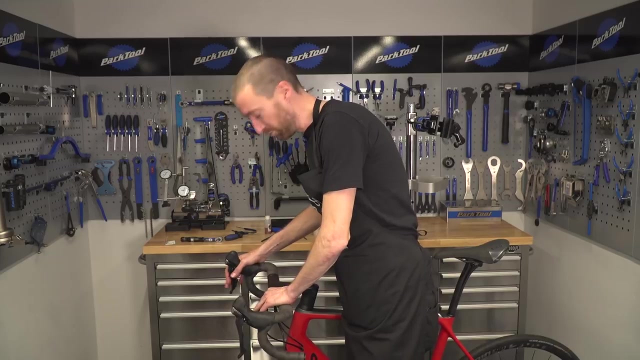 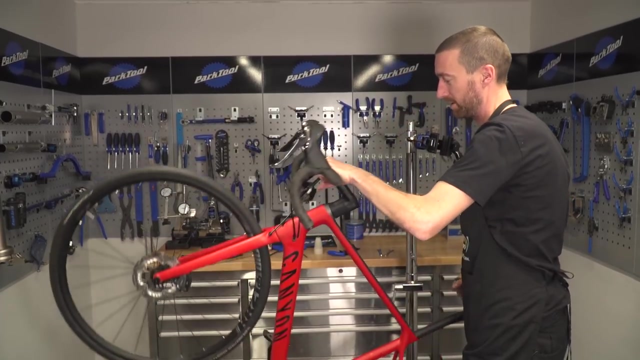 wipe over, put back on and it feels a lot more solid. now. if it is the rear brake which is feeling spongy, then when you're doing it, you can do exactly the same method. but when it comes to bouncing the bike up and down, use the gravity to your. 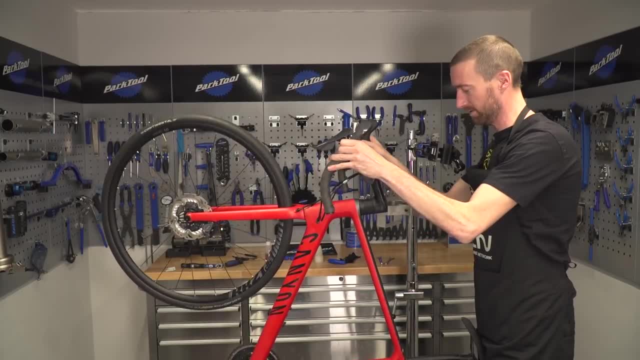 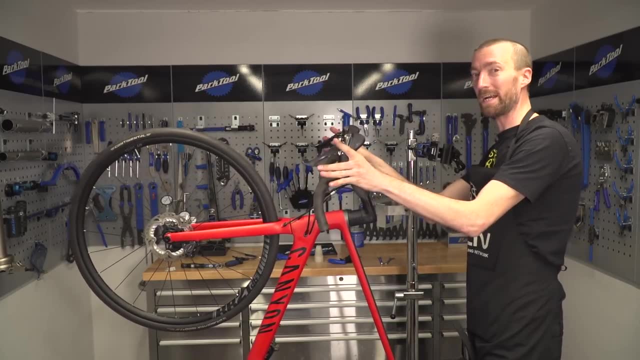 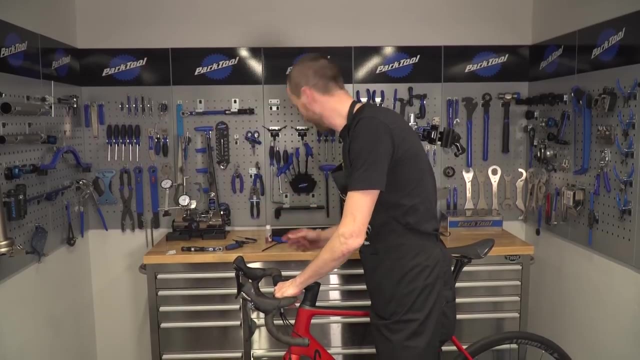 advantage. so the air comes upwards, but the bike here just bounce it gently at that point whilst pulling the brake lever on it, and those three hacks should solve a lot of your disc brake problems now. one more thing that you can try if you are finding you're getting air in this system is to focus on the points. 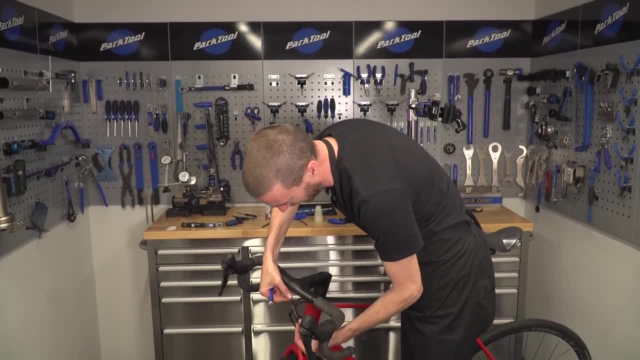 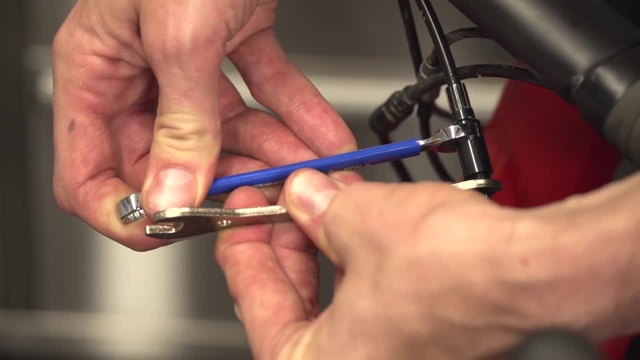 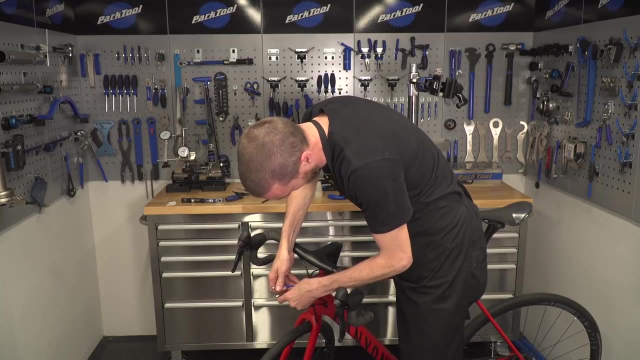 where air might be getting in. so, for example, the part here which connects two cabling parts here expose the bottom part, which normally got a rubber seal over it, and on this case it is an eight millimeter allen key there and then a nine millimeter here. and just check that these 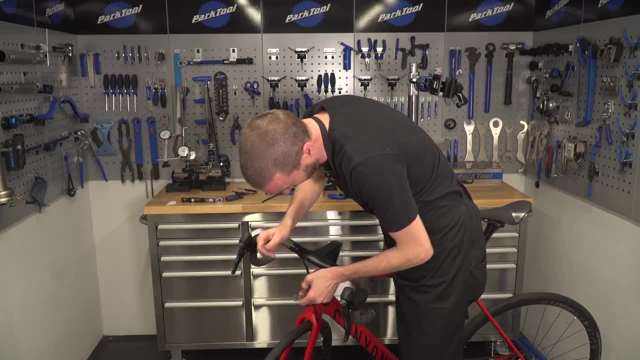 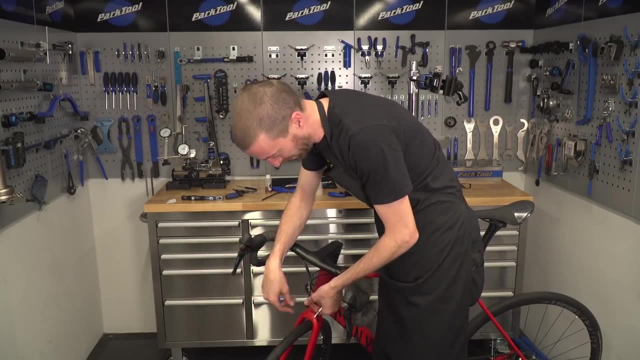 are nice and tight. you can also see whether there's any fluid around there. wipe that off of a rag, go out for a ride, because everything will still be safe, and then expose it again and see if there is any more fluid starting to leak out. and another final. 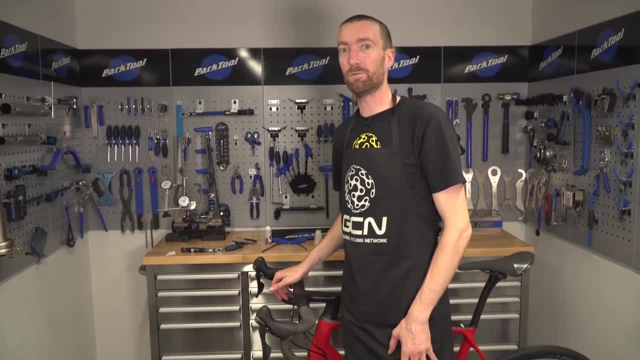 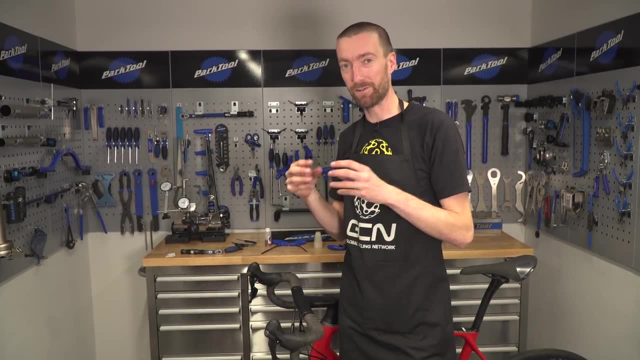 tip which you might not think about. if you're new to disc brakes, as I was a few years ago, and that is when you're traveling, you want to try and prevent the brake pads coming together and the pistons coming out. so to do that you can. 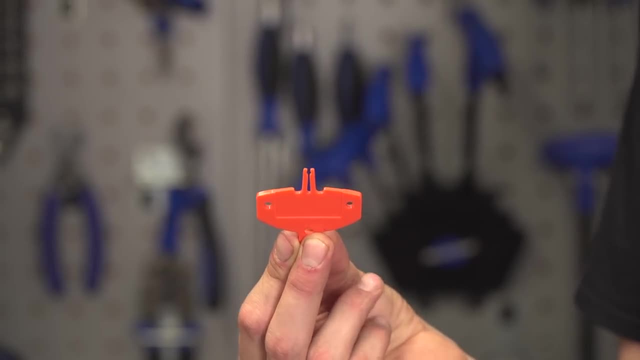 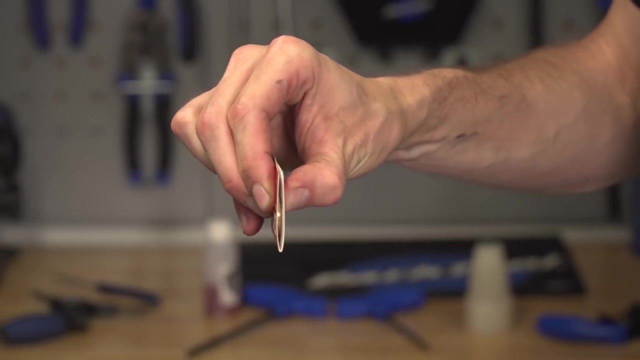 get specific spacers like this which you can put in before you go into your bike bag, or, if you haven't got one, you can simply use a couple of business cards with a very thin coin inside, and that should do the trick nicely. now we'd like: 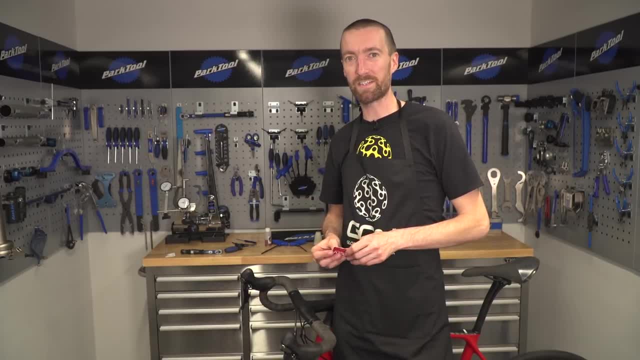 to know how you get on with all these hacks. you can do so by letting us know in the comments section down below if you'd like to see Si Richardson taking a first look at the Dura-Ace disc brake groupset a few months ago in 2017. you. 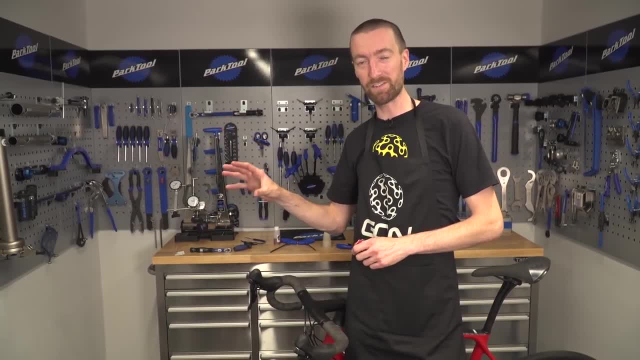 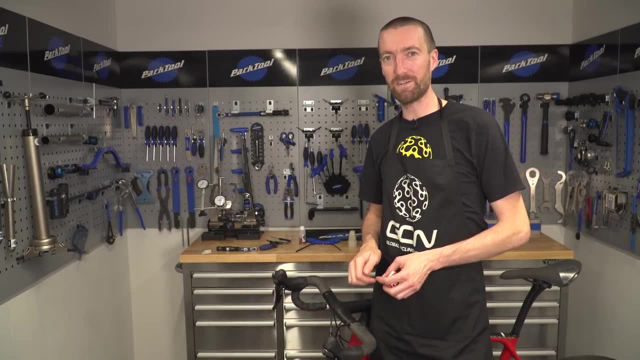 can find that in the bottom corner just down there. on the other hand, if you want 10 more general cycling hacks, you can find them in the top corner up there. and make sure you subscribe to the global cycling Network. it is free to do so. all you've got to do is click on the globe.